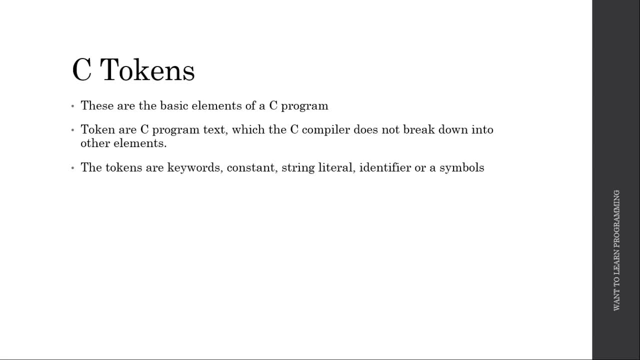 are keywords, constants, string, literals, identifiers or C tokens can also be symbols. Now let's look at some of the important symbols that are used in a C program. The first one which we will look at is a semicolon- Semicolon. 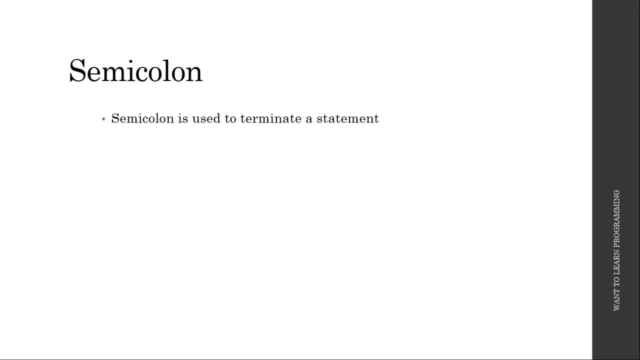 is used to terminate a statement. Now let's look at an example where semicolon is used. This is a sample program to print hello word onto the console. Here semicolon is used to terminate the statement. If semicolon is not present, then the compiler does not come to know that the statement or command has ended. 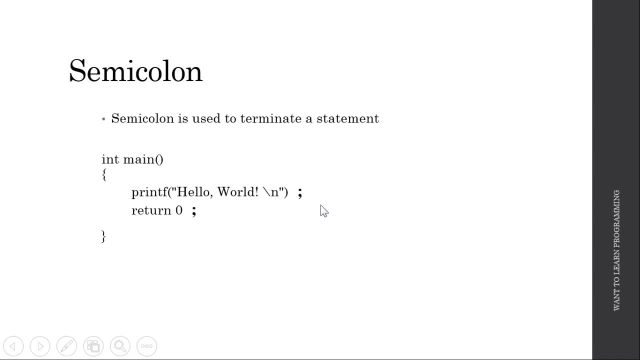 So semicolon is one of the most important piece of symbols that are present in a C program. Now let's look at what comments are. As we saw in a previous video, comments are a symbol. Comments are a group of statements which are used to make the program more reader friendly. 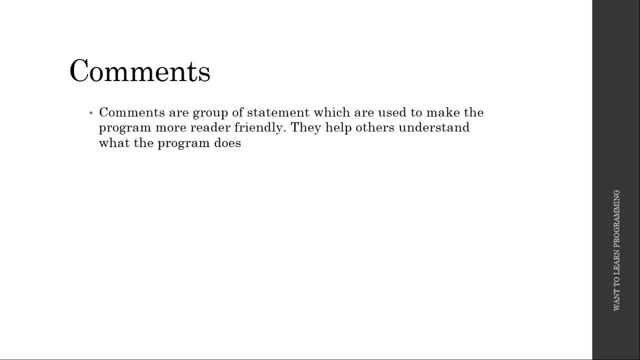 They help others understand what the program does. These comments are used when the program is complicated and a reader may not be able to understand what a statement or a block of code is doing in the program. So comments are put so that readers can understand what they are actually doing. These are ignored by the compiler, that is. 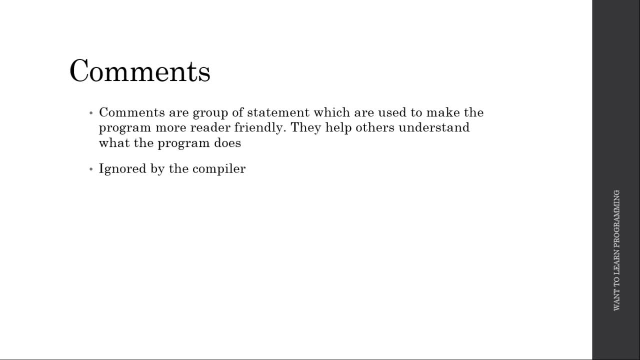 the compiler does not convert this into machine level code, so that it will not be used while executing. Now there are two kinds of comments. One is called as the single line comment and also there is something called as multiple line comment. There are two kinds of comments. The single line comment is: 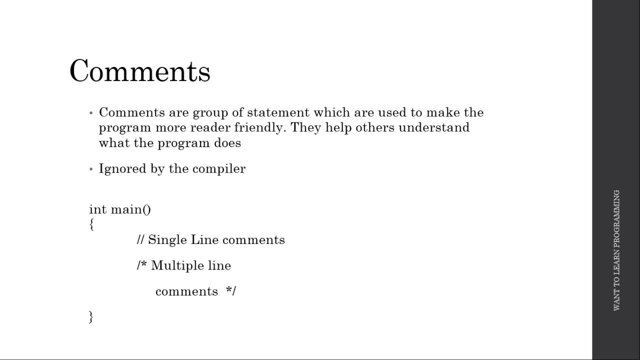 used when the comments need to be put only on the single line and they are prefixed by double slash. Multiple line comments are when you want the comments to be put on multiple lines so you can put them between a slash star and star slash sequence.